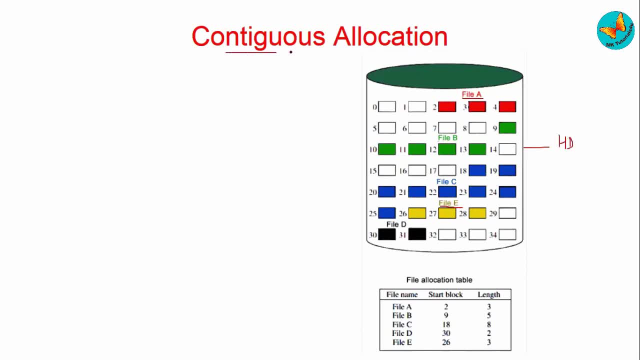 So the word contiguous means what they will be in adjacent memory location means they will be in sequence. So suppose, if I consider file A, So what the contiguous allocation means, what it does is that it will be in adjacent memory location. So the word contiguous allocation means what it does is that it will be in adjacent memory location. 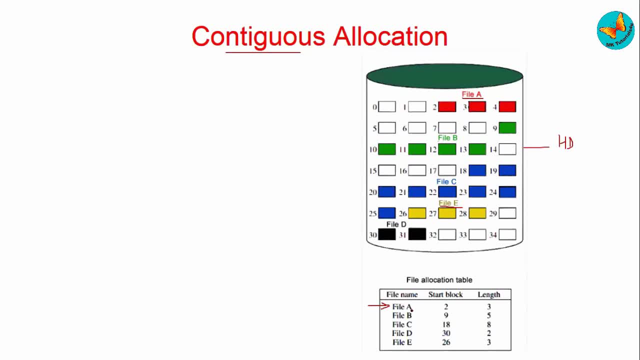 structure says is that this file A will start at the block 2, and what is the length of this file? is, say suppose, 3, then starting from the second block, it will occupy the next three adjacent blocks. means 2, 3 and 4 will be used to store the file A. Now it is not like that one block is here. 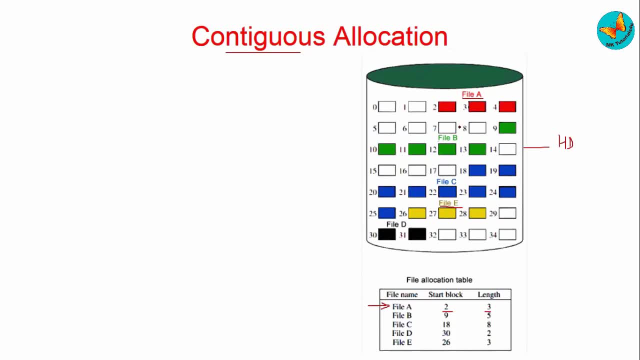 one block is there. it is adjacent because why the word is contiguous. Now consider again second example, file B. So see, here it is indicated by green color. so it starts from the location 9 and it ends at the location 13.. Why? because the length is 5, 9 plus 5. it is ending at this 30th. 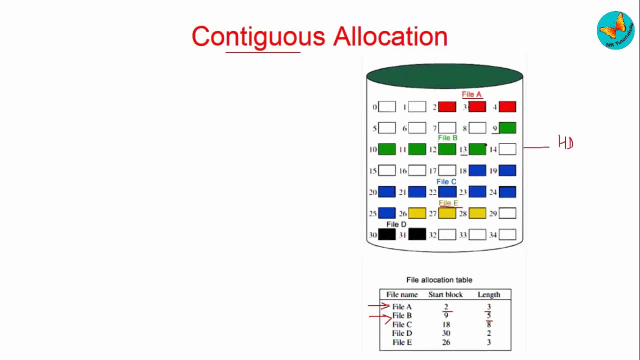 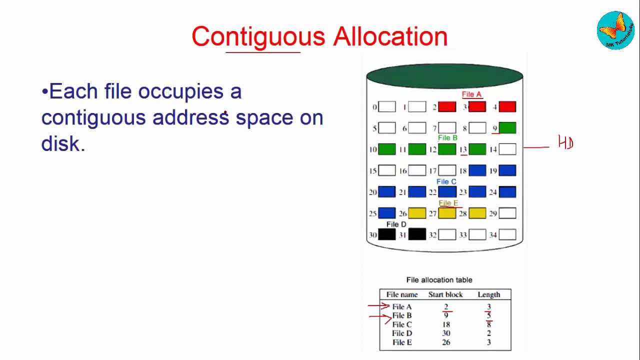 is assigned in linear order, means in increasing. linear order means: after 2 it is 3, then 4, after 9 it is 10, after 10 it is 11. so it is assigned in linear order. then it is very easy to implement. but what is the drawback of this? 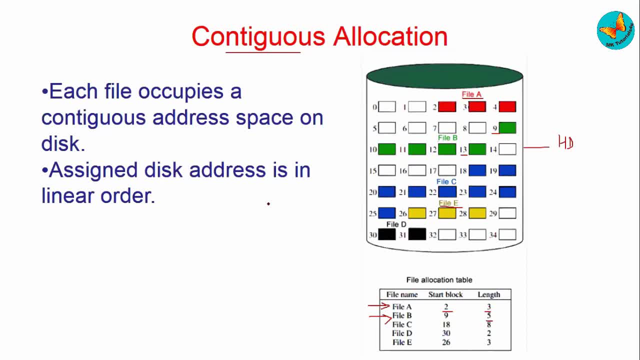 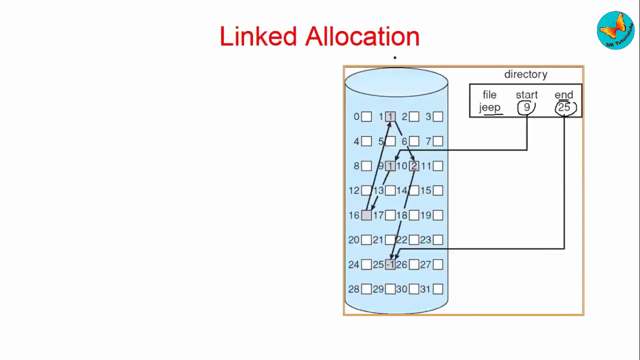 allocation is that due to this contiguous allocation, external fragmentation may occur in this allocation technique. so this is the simplest technique to allocate space for your file on the hard disk. Now let us see the second method. second is a linked allocation. So here what is happening is that now, say, suppose I have considered here one file, suppose its name is: 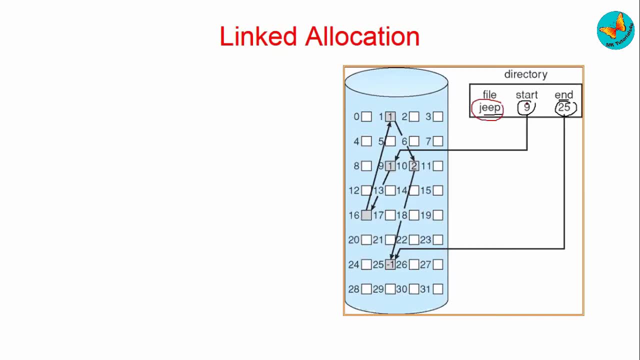 jib. so it starts at the start block is 9 and where it is ending at the block, number 25. so here what is happening is that the blocks need not be adjacent to each other like that in the contiguous memory allocation, but then how they will be linked together by this links. so 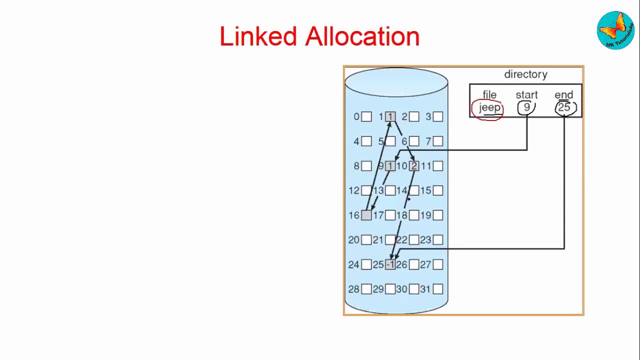 these links are used to group together all the blocks of the required file. what will happen due to this? a list of links is to be required for this type of allocation. then this directory will consist of links or pointers to the first blocks from. the first block of the file means, like it should know, that from here the first block is starting and since none. 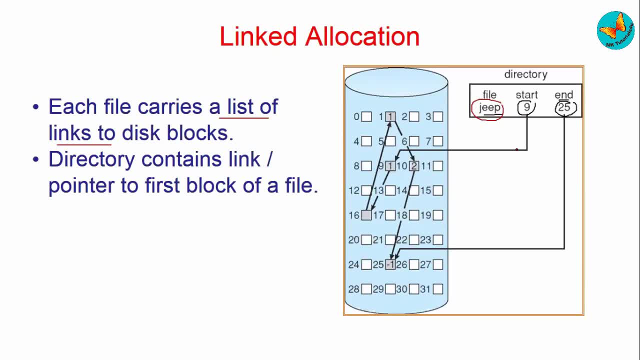 the block is wasted like that in the contiguous memory allocation, it does not suffer from the external fragmentation, and this is very effectively used in sequential access file, because in sequential access file you just have to go from one block to another block, isn't it? but then what is the drawback of this particular allocation system? is that this is inefficient. 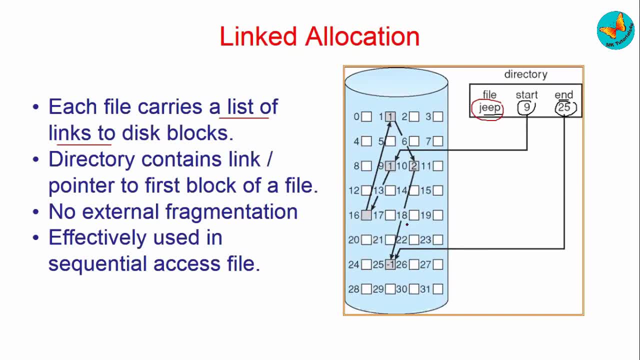 when you want to direct access the file means, say suppose, if i directly want to go a particular block. so that is not possible in this type of link allocation. so we have seen some advantages and disadvantages of the two types of allocation. now to overcome this disadvantages we will see the last allocation, that is, the indexed allocation. 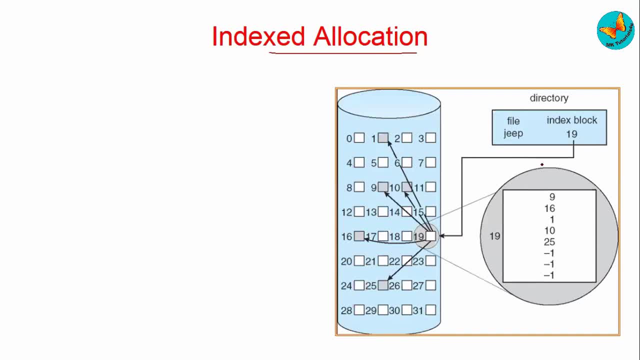 now you observe here, here again the file zip is taken and here first the index block is kept and within that index block all the pointers to various location of the disk blocks are kept. means, say suppose here this consists of nine numbers: 16, 1, 10 and 25 number of blocks for storing. 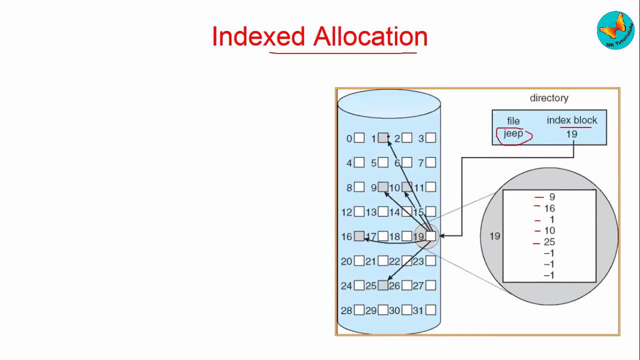 in a particular file and, due to this, what is happening is that, see, what was the drawback in contiguous memory allocation? it was suffering from external fragmentation, isn't it? and and what was the drawback of this link allocation it was suffering from is it could not directly access the 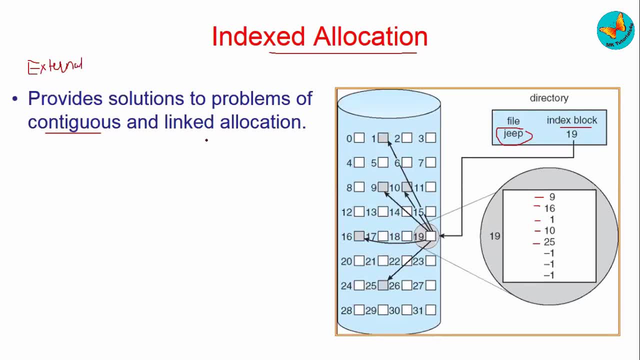 direct access file, isn't it? these were the drawbacks, so the index blocks are overcome in this index allocation. so what is happening here is that a index table is maintained, like i have shown you here. then it easily enables us the random access which was not possible in link allocation. and then this index blocks consist of all the pointers to 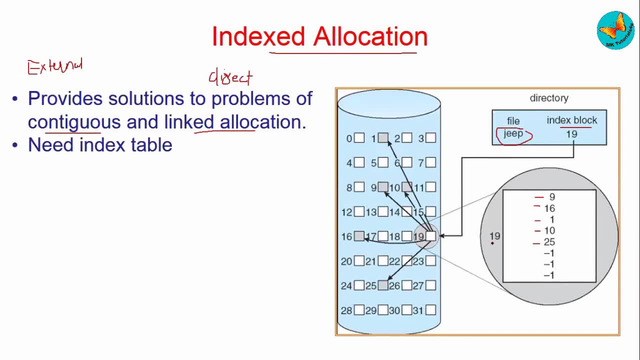 the files, and then each file has its own index block which stores the addresses of the displays. so like here. i have taken one example of this file, jeep, and here for that jeep file the index block is there. so, similarly, for every file, such type of index block will be created and within this index 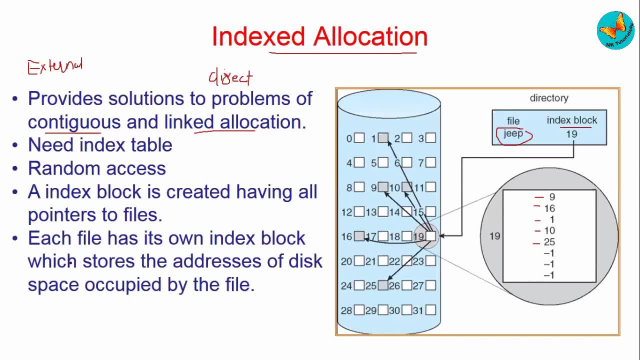 block, there will be pointers to the files. so, due to this, what is happening is that this directory will consist of the addresses of index blocks of the files, means in a particular hard disk, multiple of the file could be there and for each file, then for each file, index block will be created and that 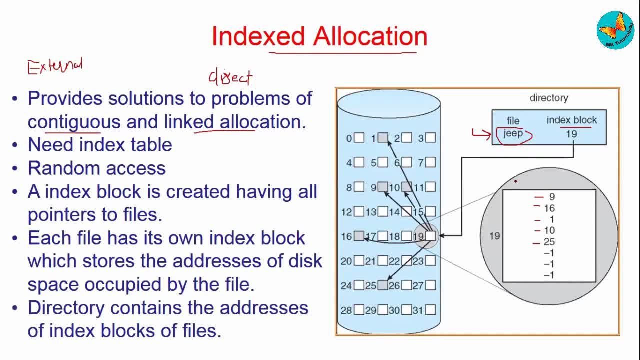 will be stored within the directory. so this index allocation overcomes the disadvantages of both the contagious allocation and the link allocation. so mostly this is preferred over contagious and the link allocation. so once again i'll repeat this: from external fragmentation, because their memory is wasted, and in link allocation what is happening. 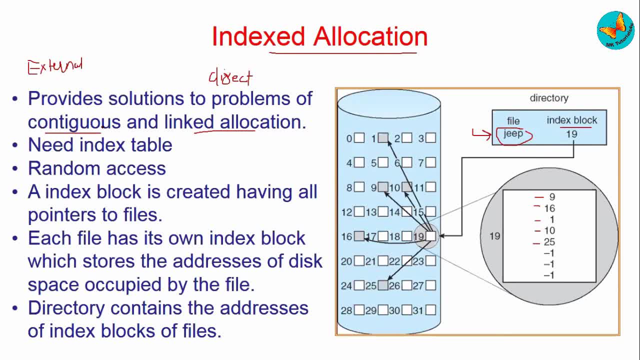 is that you cannot use this on direct access file. So both these drawbacks are overcome by creating an index table and for every file one type of block is created that is known as the index block and which consists of the pointers to various disk block within a particular file.